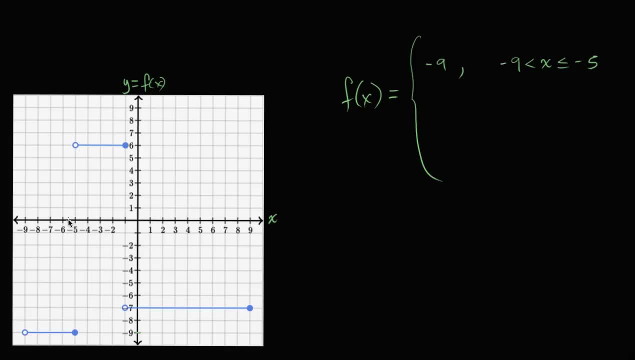 But now let's look at the next interval. The next interval is from: x is greater or negative, five is less than x, which is less than or equal to negative one, And over that interval the function is equal to. the function is a constant six. It jumps up here: 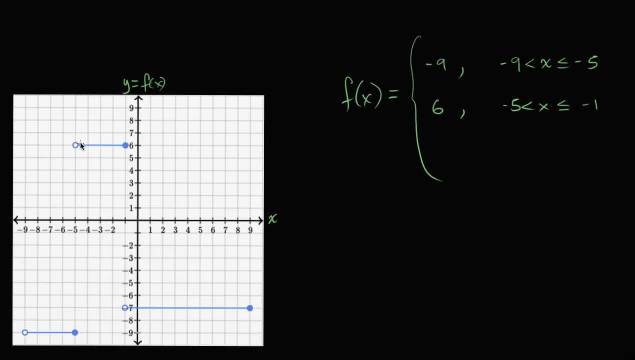 Sometimes people call this a step function. It steps up, It looks like stairs to some degree. Now it's very important here that at x equals negative five for it to be defined only one place Here. it's defined by this part. It's only defined over here. 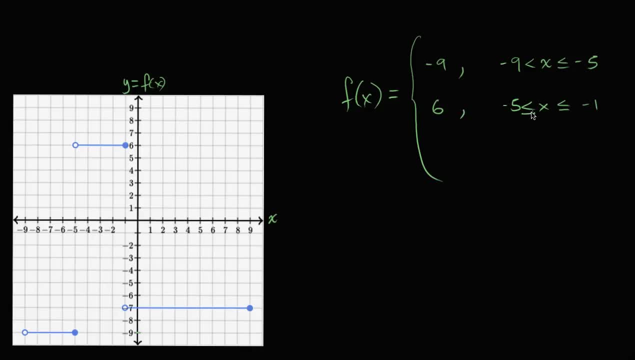 And so that's why it's important that this isn't. a negative five is less than or equal to, because if you put negative five into the function, this thing would be filled in, and then the function would be defined to both places, and that's not cool for a 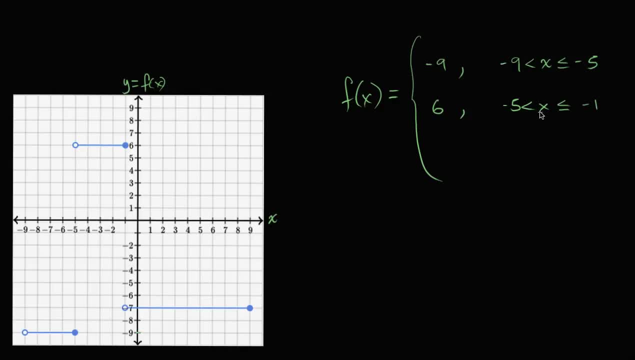 function. It wouldn't be a function anymore. So it's very important that when you input negative five in here, you know which of these intervals you are in. You can't be in two of these intervals. If you are in two of these intervals, the intervals should. 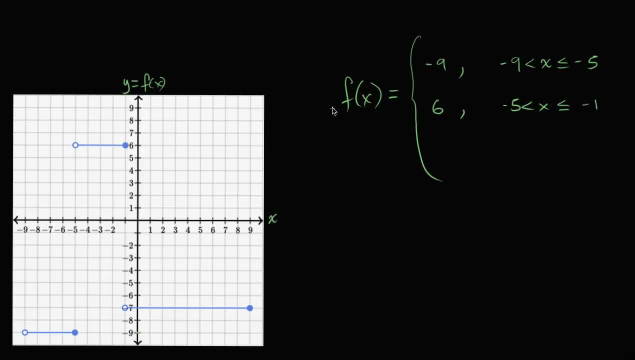 give you the same value, so that the function maps from one input to the same output. Now let's keep going. We have this last interval. we're going from negative one, we're going from negative one to nine, From negative one to positive nine, and 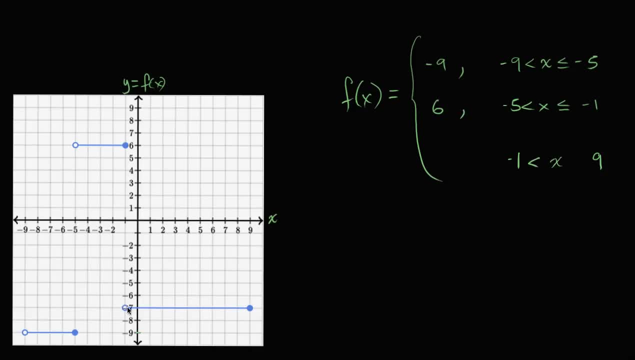 x, it starts off with negative one less than x, because we have an open circle right over here. That's good, because x equals negative one is defined up here all the way to. x is less than or equal to nine. and over that interval, what is the value of our function? 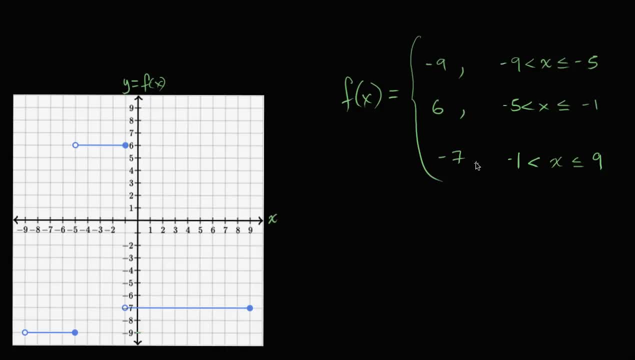 Well, you see, the value of our function is a constant negative seven. a constant negative seven. And we're done. We have just constructed a piece-by-piece definition of this function And actually when you see this type of function notation, it becomes a lot clearer why function notation?